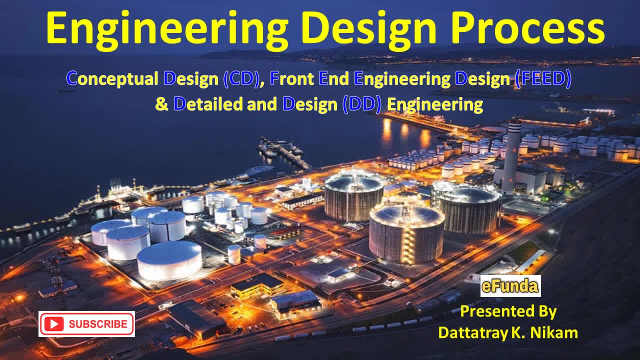 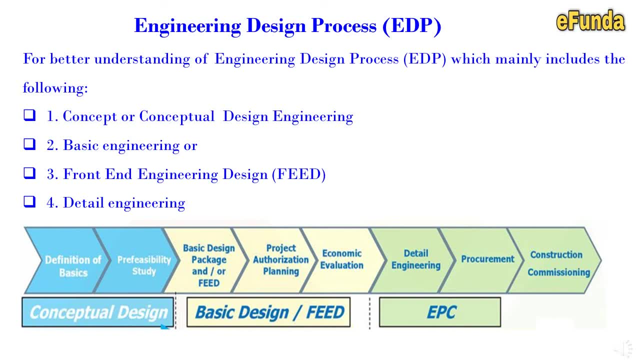 So please do subscribe to our channel and watch the video created on the introduction to engineering and project, which we have already created and produced below figure, where we have aggregated conceptual design, basic feed design, EPC, where conceptual design consists of definition of a basic free feasibility study in basic design, basic. 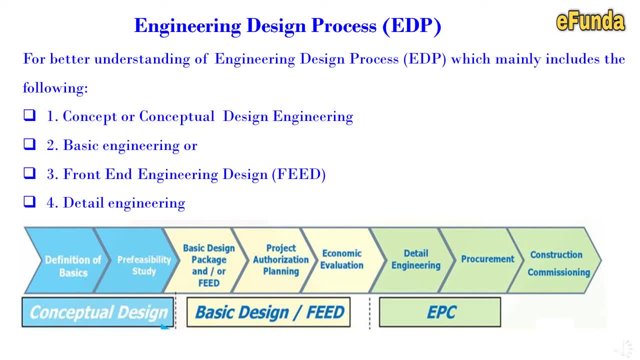 design package or a feed project, authorization planning, economic evaluation under EPC, detail engineering, procurement, construction and commissioning. These are the phases, which include. various stages of engineering are depicted in the picture. For further detail, we will move on to the next slide where we will cover each topic. 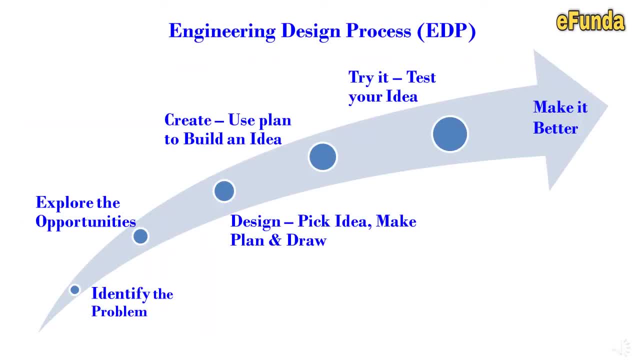 in detail. Engineering design process can be understood from the sketch below, where we have identified each point for better understanding. We will start with identify the problem, explore the opportunities where we can improve on your identified problem, Then design, that is, pick your idea, make some plan and then draw accordingly. 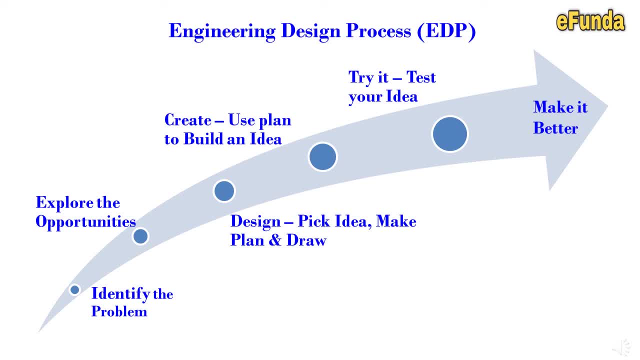 Then create. that is, use your plan to build an idea which is there in your mind. Again, try it out. that is, test your idea to implement and, after implementation, make it better how you can improve and implement the idea which you have in the beginning. or 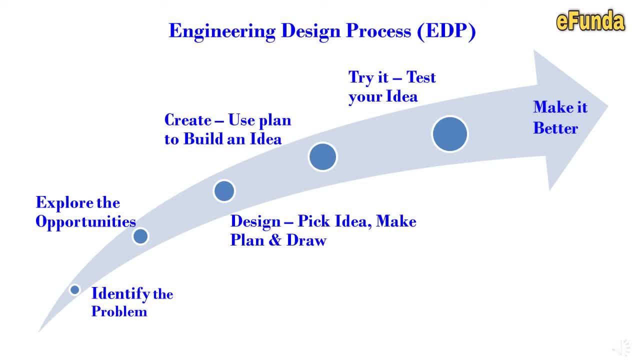 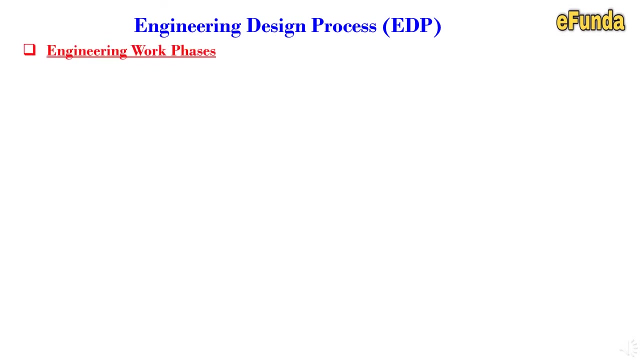 which you cannot implement. This is how engineering design process helps to understand the complete process of any project or objective which are there in your mind and with this approach you can simplify it before implementation of any idea or any project which you have. Moving on to engineering work phases, one can see in a below table we have identified. 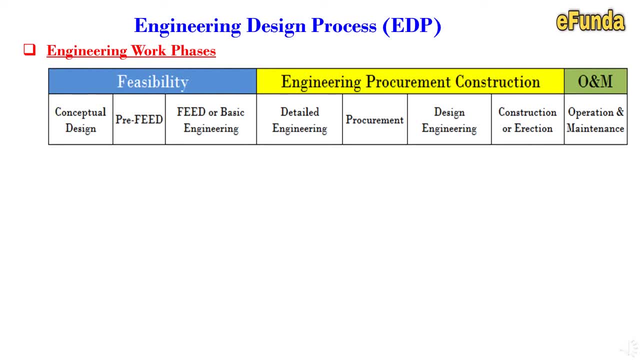 the engineering work phases, that is, the feasibility- the feasibility of the project, the feasibility of the project, the feasibility of the project and the feasibility of the phase- and are none of the preliminary procedures Under feasibility. EPC, that is, Engineering Procurement and Construction team, is responsible. for the outlook of what the project can look like. so On-Site Problem Analysis Group and I, Inspector, Up 들어가ed with their approach and the auction of this process. encant Duomo estran, known to you, can go to. O Choose the. 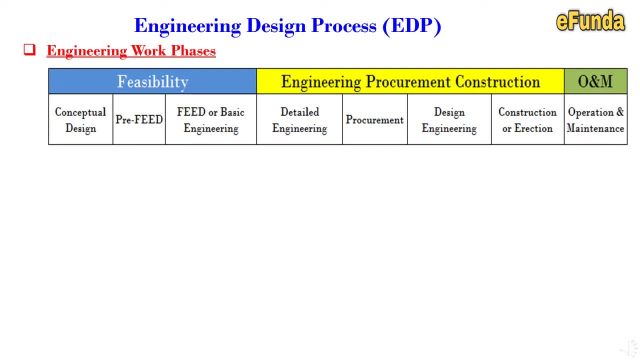 box under feasibility. EPC, that is Engineering Procurement and Constructionminute Before Washington. Lee Namban, I нож into one aspect: O and M, that is Operation and Maintenance. Under feasibility, we have categorized conceptual design, pre feed or basic engineering under 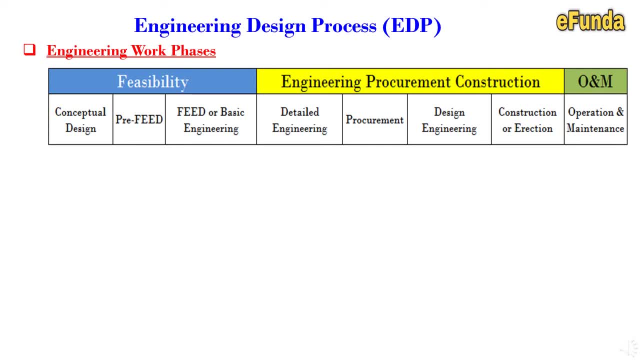 EPC detail engineering, procurement, design, engineering, construction or ere stationed and on the on the here the dataierung process and plan review. Go to the explaining definition below the video link and go to the description below: 졌лон должна uta 우ies waterfall. 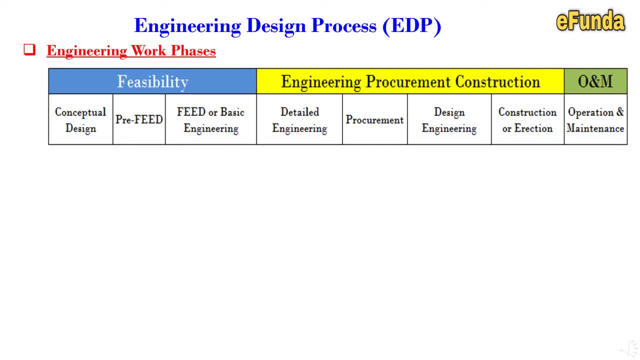 With this. this is how the engineering work phases are divided, each organization based on their work procedure methodology. various stages are being carried out as part of the engineering design where this concept are being employed, based on the tech scope. Scope may be vary, stages naming may be vary, but the work done under these stages will remain. 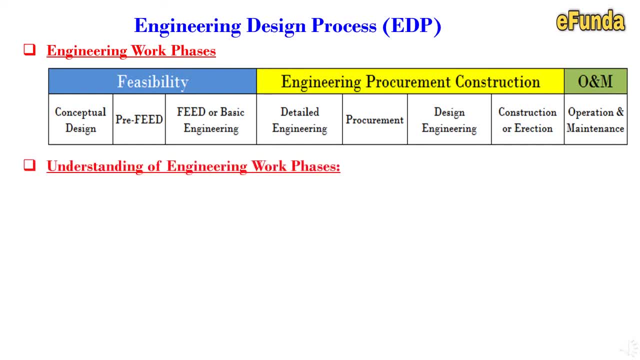 based on the project scope. Moving on to understanding of engineering phases, we will see the feasibility. This is an assessment or evaluation of a proposed plan or a method or a new project, that is, a defined objectives or goals. This involves study of the legal economic technology. 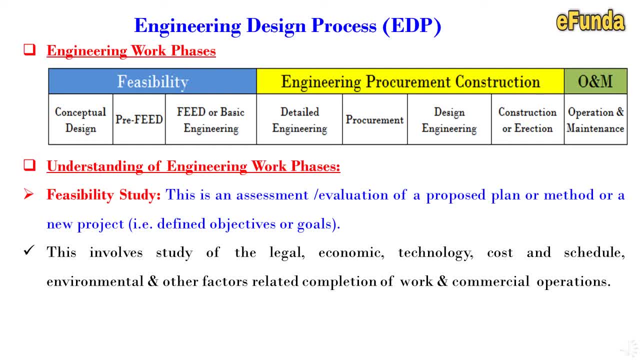 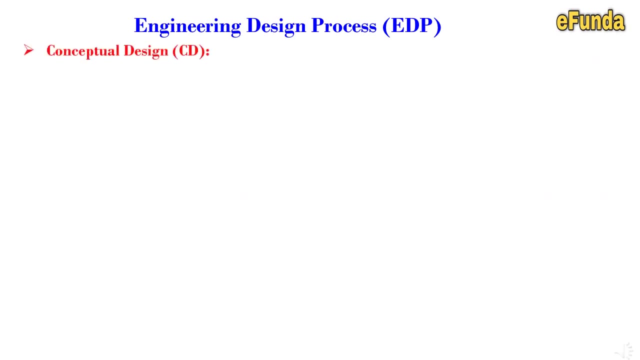 cost and schedule, environmental and other factors related completion of a work and commercial operation In general. the feasibility study is a preliminary study performed in the early stage of the project. A conceptual design or speed engineering stage will be followed. Conceptual design, that is, a CD. This is an initial design document for the initial design. 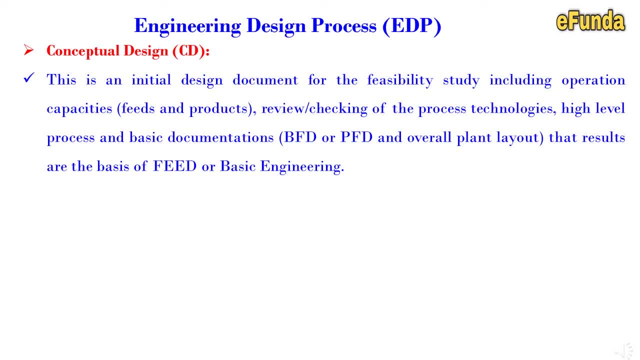 feasibility study, including operation capacities- that is, feed and products- review, checking of the process, technologies, high level process and basic documentation is a bfd or pfd, and overall plant layout. that results are the basis of feed or basic engineering. this stage of a project is done to minimize the likelihood of error, manage cost, assess risk and evaluate the potential success. 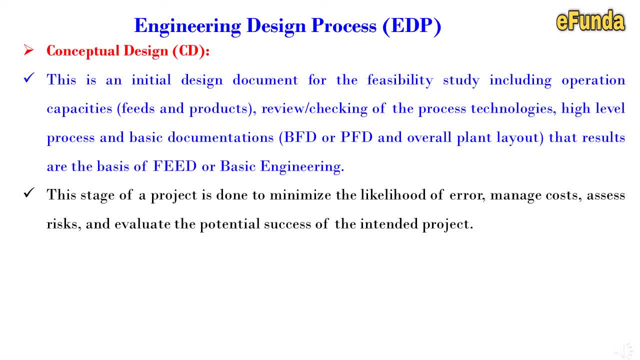 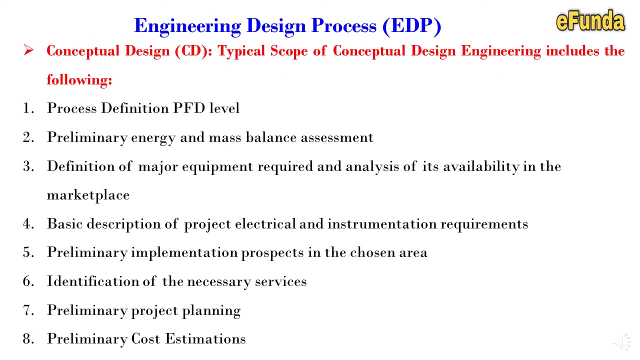 of the intended project at the conceptual design stage decide. that is, a plant location selection study, initial project schedule- that is level one- and a budget cost estimation, factorized estimated in the range of maybe 42 plus minus 100 percent, can be performed together. conceptual design: typical scope of conceptual design engineering includes the following: 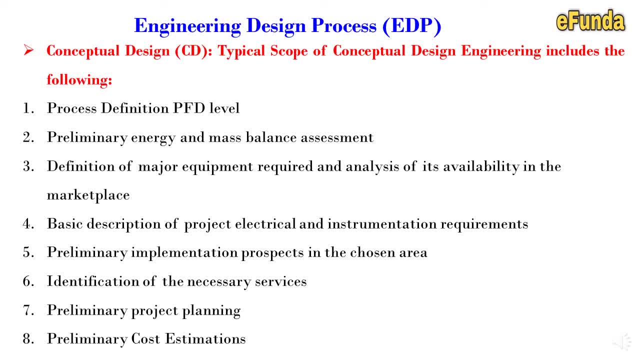 process definition. tfd level. preliminary energy and mass balance assessment. definition of a major equipment required and analysis of its availability in the market place. basic description of a project: electrical and instrumentation requirement. preliminary implementation prospect. design the chosen area. identification of the necessary services. preliminary project planning. preliminary 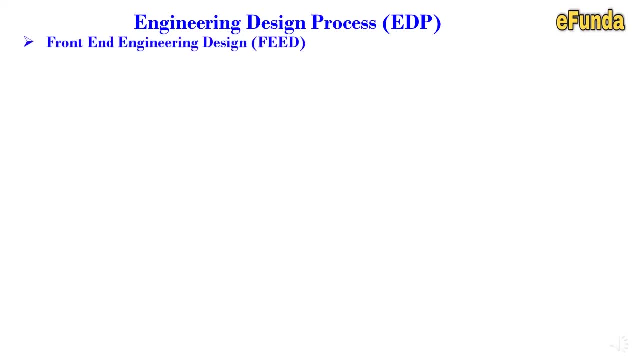 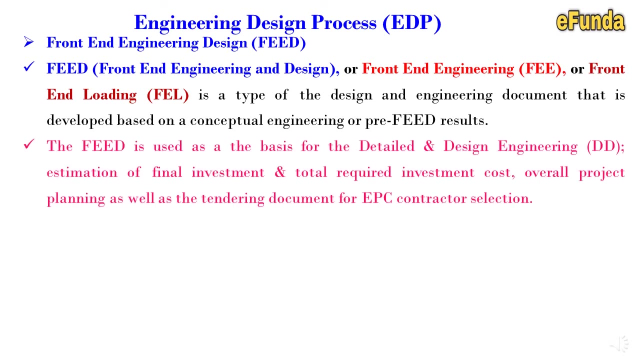 cost estimation. front-end engineering design- that is a feed. front-end engineering design or front-end engineering- that is fee or front-end engineering loading- that is fel is a type of design and engineering document that is developed based on conceptual engineering or pre-feed result. the feed is used as basis for detailed and design engineering. that is a dd. 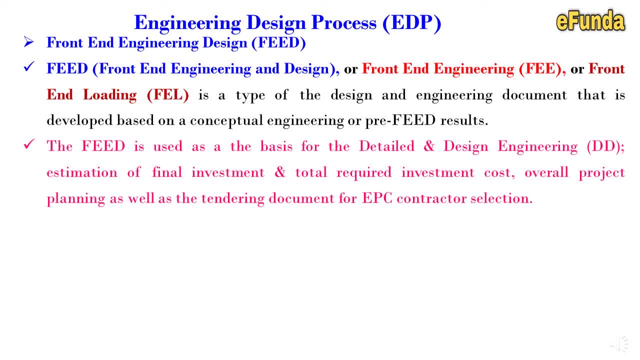 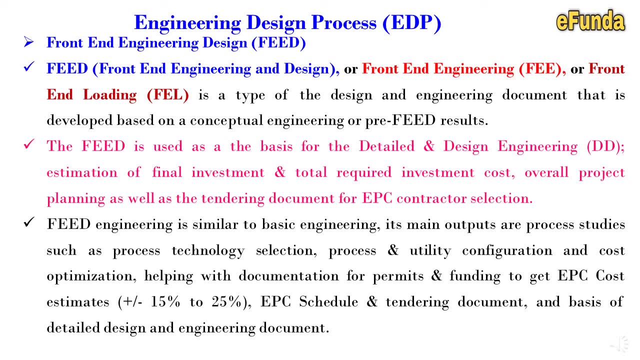 estimation of final investment, total required investment cost, overall project planning, as well as the tendering document for epc contractor selection. feed engineering is similar to basic engineering. its main output are: process study, such as a process technology selection, process configuration and cost optimization. helping with the documentation for permits and funding to get. 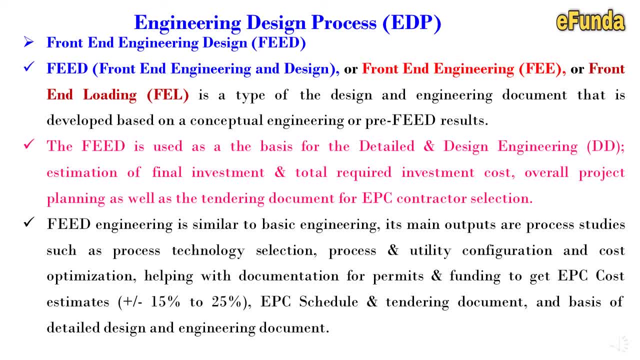 epc estimate in the range of plus minus 15 percent to 25 percent. epc schedule and tendering document- the basis for detail, design and engineering document. this is how the feed is defined and used for the purpose of detail and design engineering, for better understanding of front-end. 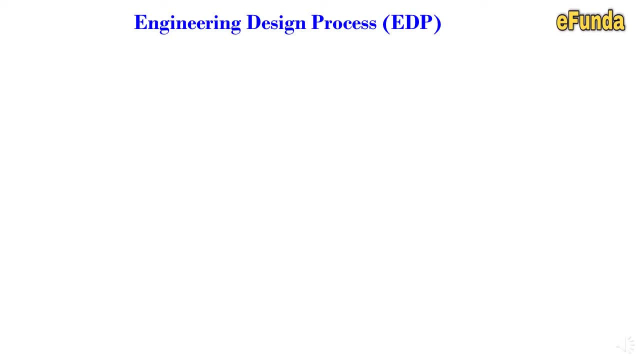 engineering design. that is a feed which requires to have an understanding on feed process. one can see in a below figure where feed planning, data collection, basis for design, field estimate, final documentation. these are the stages one should understand under field planning one will define that how the project is planned and what is the 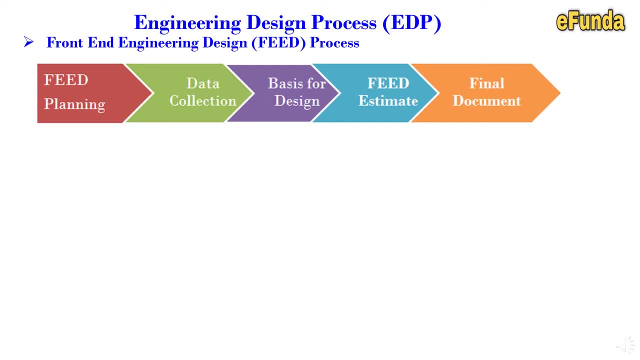 planning and what is the schedule you have made it to execute this. and the data collection is where, if you are doing the modification or updating the existing facility, then the details of existing equipment, their plant layout and required details to be captured as part of the site survey. 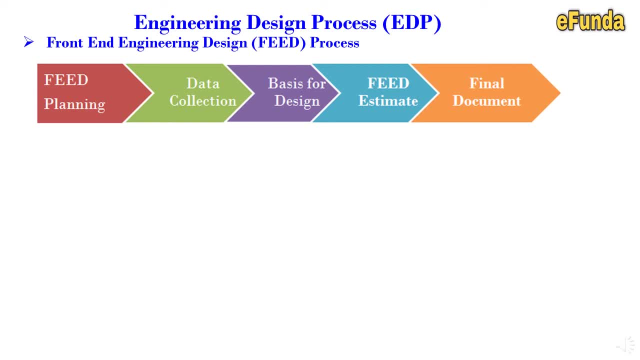 which falls under the data collection for proper execution of the plan basis for design. you should have a complete design basis where: what is the scope, what are the requirements of the project scope, what is the objective to be achieved, what is the cost estimate and what is the design. 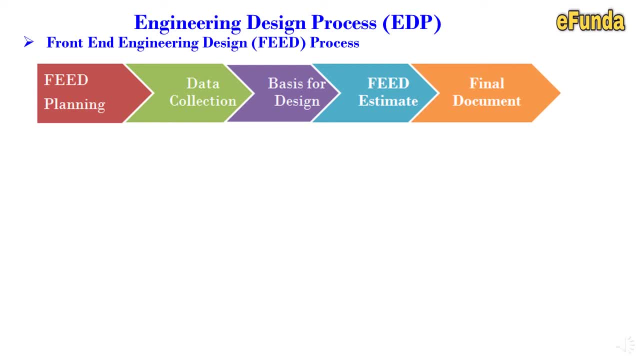 consideration to be considered for this: design: speed estimates, which involves the estimation requires the details of overall project, typically techno-commercial feasibility to narrow down the cost and the benefits for overall estimation of the project, which mainly includes detail: functional scope of the engineering design project plan, detail procedure plan final documentation. the feed final document is definitive technical. 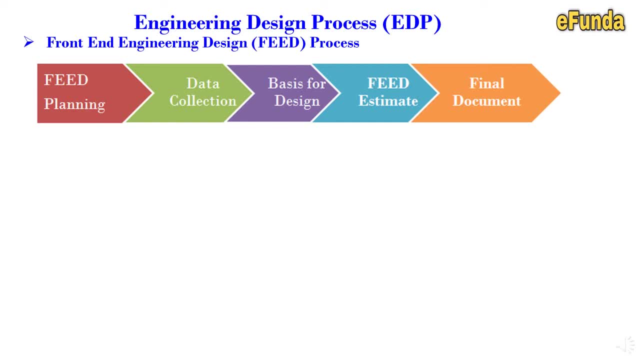 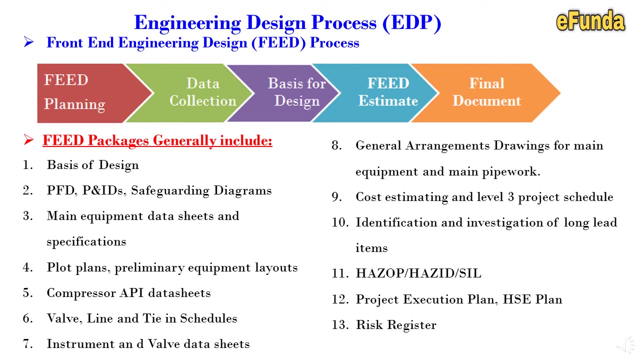 and business project summary, which includes all the deliverables produced by the organization while executing the project, and these are definitely includes the documents like project scope definition, project execution plan, economic justification. this is the about the feed process. now, feed package generally include other equipment related information, like the: 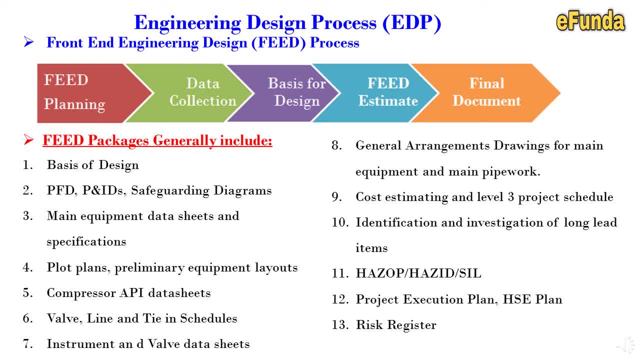 first stage of construction and the first stage of construction. so these are the main items which are included in the plan basis of design: cfds, cnids, safeguarding diagram, main equipment data sheet and specifications. plot plans play with preliminary equipment layout, compressor, api data sheet, valves line and time schedule instrument. and. valve data sheet: general arrangement drawing for main equipment and main pipe, rack cost estimating and level 3 project schedule identification invest deeply and the blend method is for the main equipment and main pipe rank cost estimating and level 3 project schedule identification, in which design is also included in the plan basis of design. a 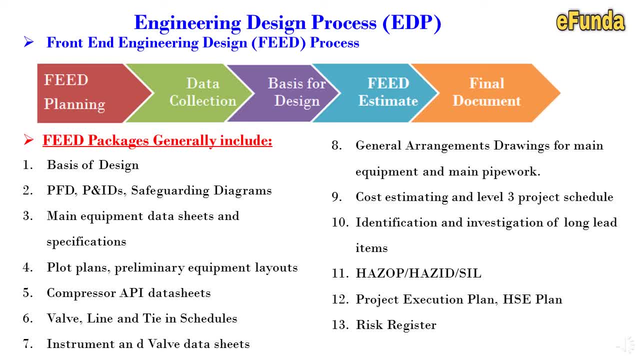 of a long-lead item: HAZOP HAZID, TIL studies project execution plan. HSC plan, RASC register. These are the few deliverables should be part of the field package while delivering or submitting to the client for their further tendering and EPC contractor selection. 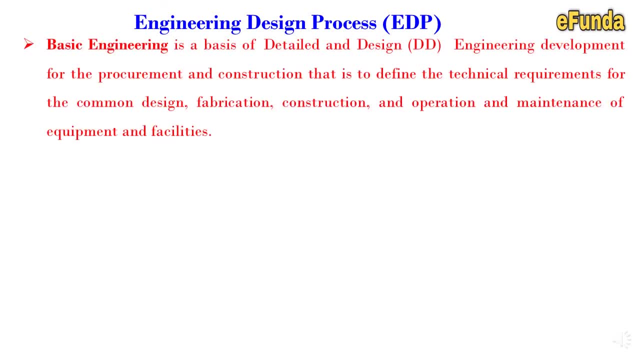 Basic engineering is a basis of detail and design engineering developed for the procurement and construction, that is, to define the technical requirement for the common design, fabrication, construction and operation and maintenance of the equipment and facilities designed for the to build Cost estimate. the basic engineering phase may typically be reduced. 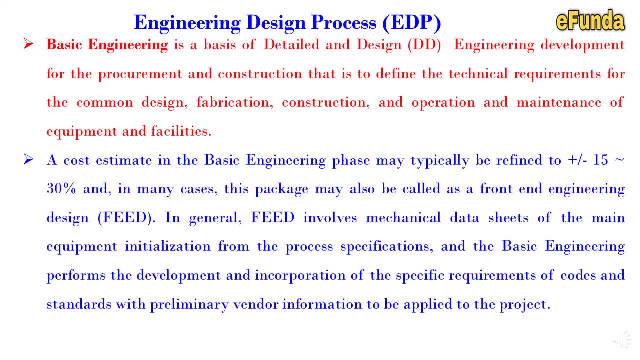 Defined to plus minus 15 percent to 30 percent and in any cases this package may also be called as a front-end engineering design, that is, a feed In general. feed involves mechanical data sheets of the main equipment, initialization from the process specification, and the basic engineering performs the development and incorporation. 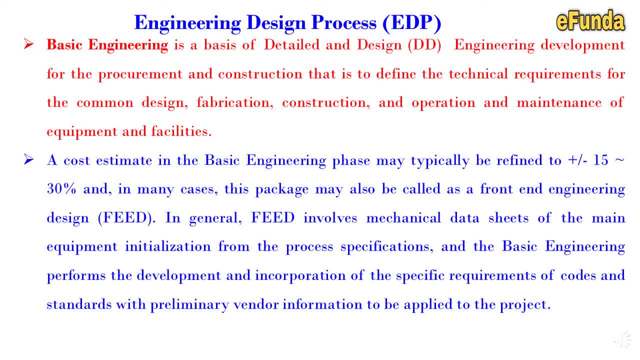 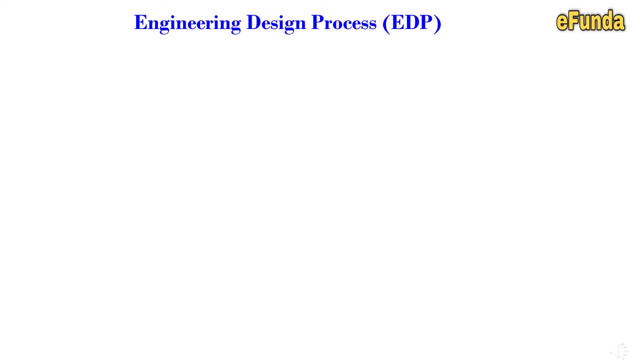 of the specific requirements of the codes and the standard with the help of preliminary vendor data information to be applied. Detailed engineering: detailed engineering is the complete project implementation, from an engineering study to starting a particular plan, including layout, drawing, analysis, procurement, construction and finally leading to commissioning of a build facility. 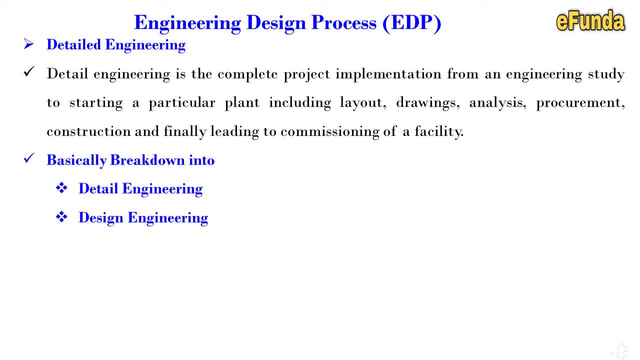 Basically this breakdown into detail and design engineering, that is, a DD. detail engineering is the complete project implementation, From engineering study to the final design and commissioning output of this facility. as a process build up, This study ensures that multi-discipline performs their work and complete defined interfaces. 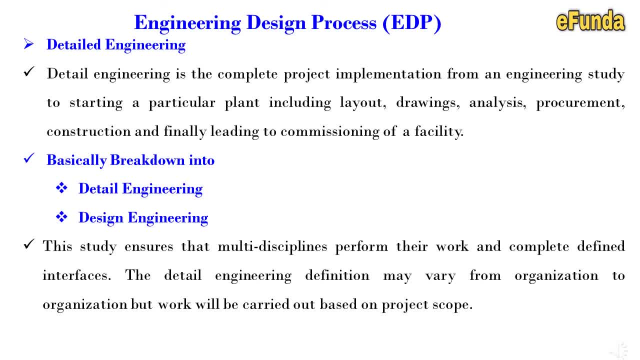 The detail engineering definition may vary from organization to organization, but work will be carried out based on the project scope Under detail engineering. The detail engineering is worked out by the engineer for preliminary estimations, as well as including their involvement in the procurement of the activities and, basically, the implementation. 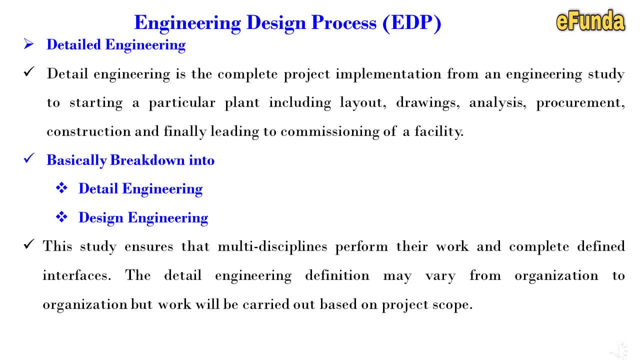 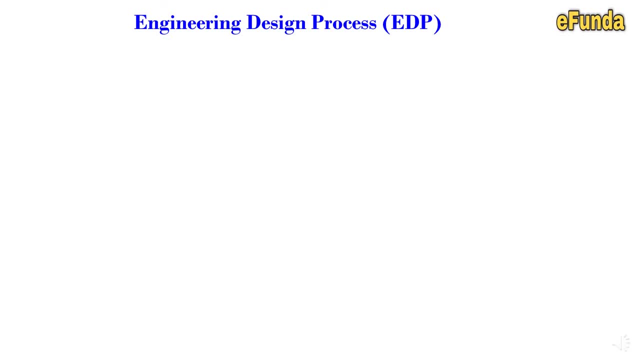 part that is the construction engineering. that is part of the design engineering, where all the layouts, drawing, hookup, loop drawing, wiring diagram, implementation, structure, setup. these are the part of the design engineering As part of detail engineering. Detail engineering includes the following function: that is the technical description. 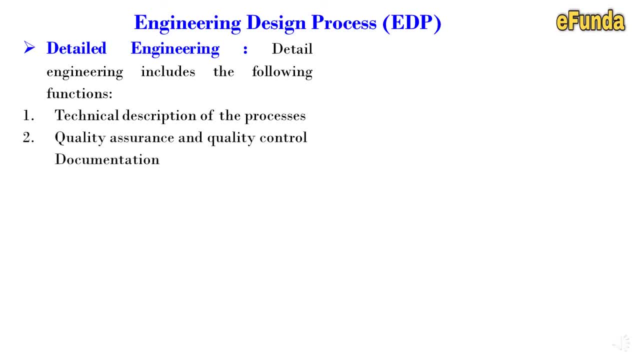 of the processes. second, quality assurance and the quality control documentation. use of computer aided engineering, that is, CAE tools: layout, planning and detail coordination. clarification of the details. design of the pipe, layout and instrumentation, calculation of a material requirements and technical specifications, definition of interfaces, configuration and. 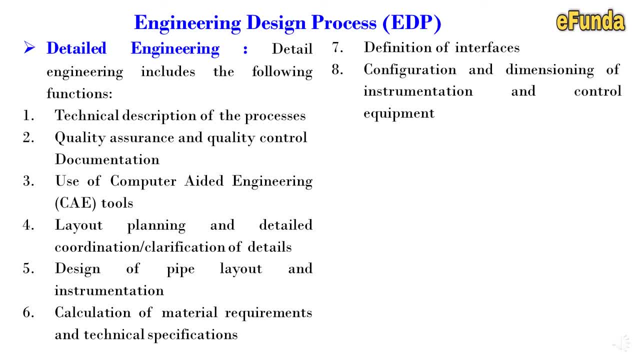 dimensioning of the instrumentation and control equipment. arrangement of a component inventory. taking on to the site. monitoring of a time schedule. cost control. supervision of a construction and installation work. commissioning of a plant component supervision of a commissioning. 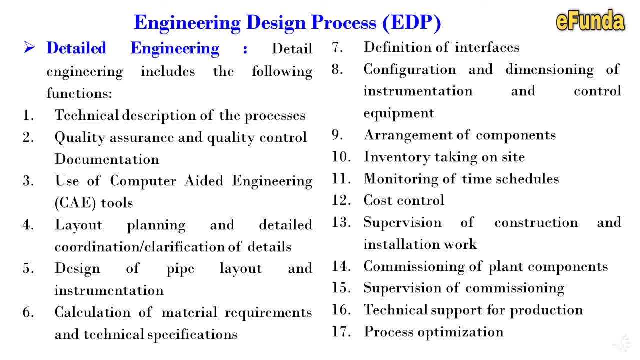 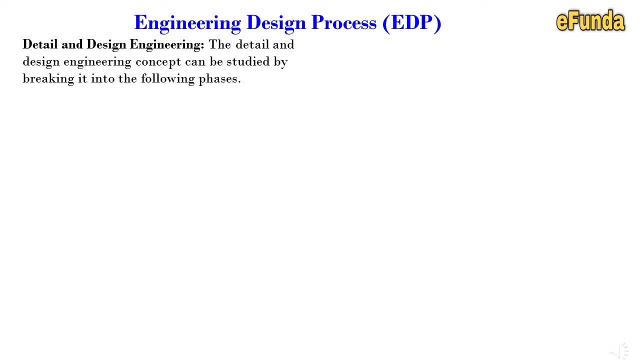 technical support for production and, finally, to the process optimization. These are the typical functions are to be considered in detail engineering phases of the project. Detail and design engineering. the detail and design engineering concept can be studied by breaking it down to the following phases: definition, scope and project execution plan. 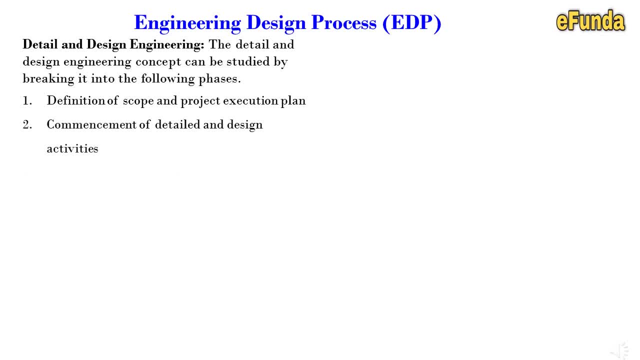 commencement of the detail and design activities: Initial design development and identification of hazard. actual design development engineering. initial design review and audit. that is 30%, 60% and 90%. design review approved for design: that is AFD approval for construction, that is AFC. design engineering. closeout detail: 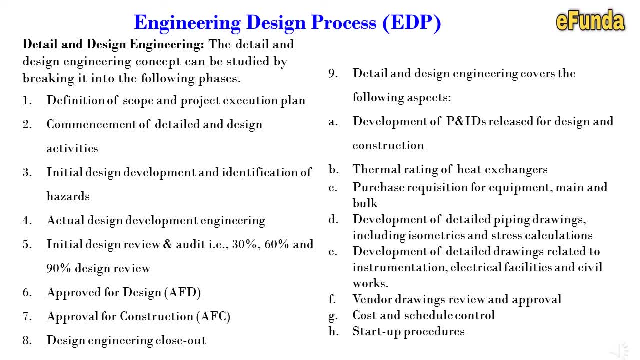 and design engineering covers following aspects, that is, development of P&IDs release for design and construction. thermal rating of heat exchanger. purchase requisition for equipment, main and bulk items. development of a detail piping drawing, including isometric and stress calculation. development of detail drawing related to instrumentation, electrical facilities.